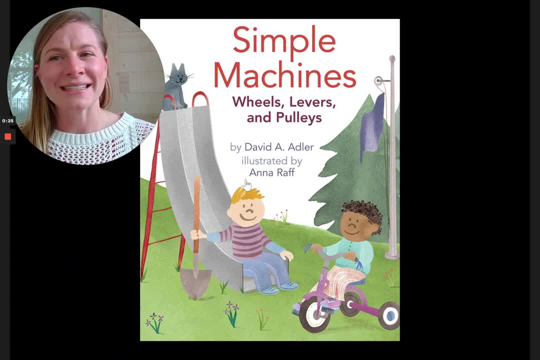 that's just a thing. But when I learned exactly how these machines help us do work, I was like: oh, these truly are the simplest forms of machines. So here we go. Let's read all about it: Simple Machines, Wheels, Levers and Pulleys. It's by David A Adler, my favorite science guy. 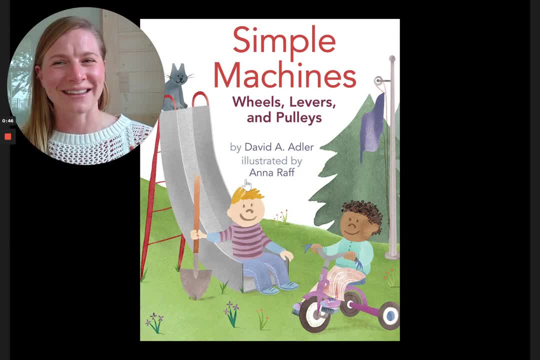 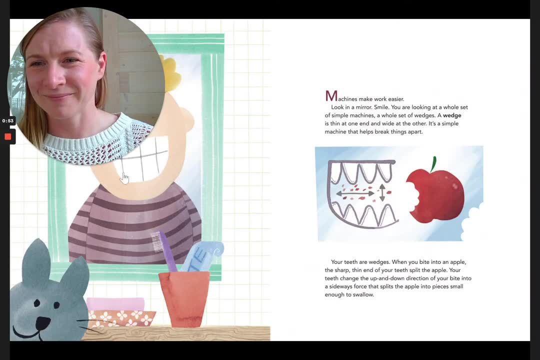 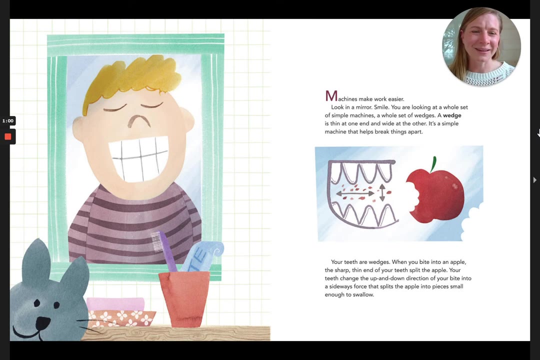 and illustrated by Anna Raff, my favorite science illustrator. Here we go, friends. Machines make work easier. Look in a mirror, Smile. You are looking at a whole set of simple machines, a whole set of wedges. A wedge is thin at one end and wide at the other. It's a simple machine that helps break things. 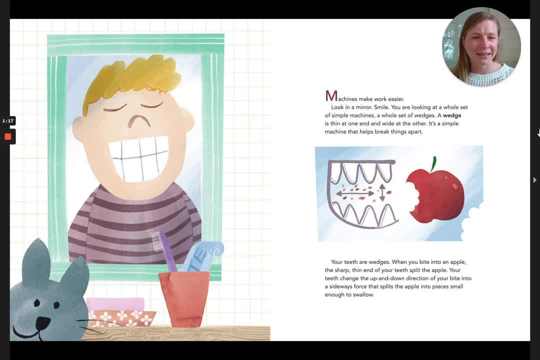 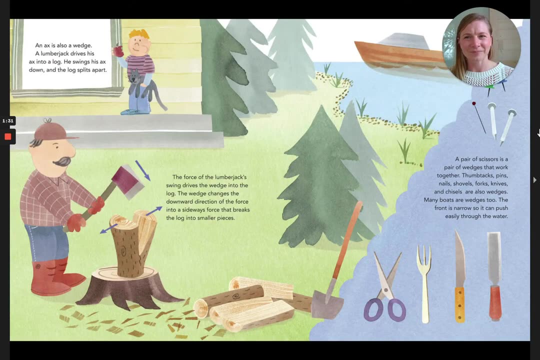 apart. Your teeth are wedges. When you bite into an apple, the sharp, thin end of your teeth split the apple. Your teeth change the up and down direction of your bite into a sideways force that splits the apple into pieces small enough. An axe is also a wedge. A lumberjack drives his axe into a log. He swings his axe down and the log. 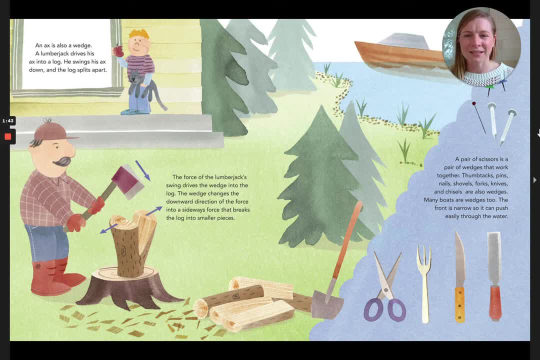 splits apart. The force of the lumberjack swing drives the wedge into the log. The wedge changes the downward direction of the force into a sideways force that breaks the log into smaller pieces. A pair of scissors is a pair of wedges that work together: Thumbtacks, pins, nails, shovels. 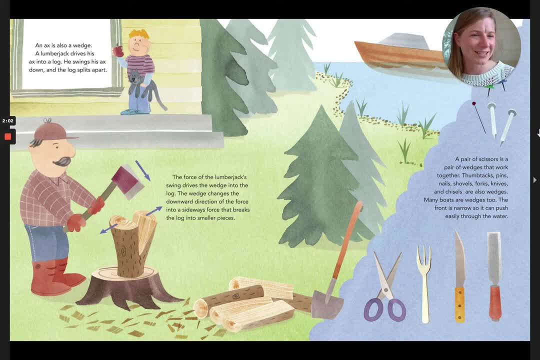 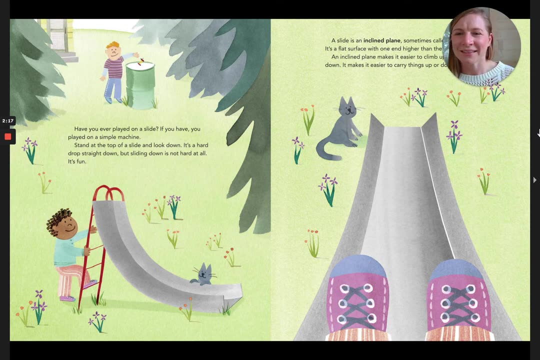 forks, knives and chisels are all also wedges. Many boats are wedges too. The front is narrow, so it can push easily through the water. Have you ever played on a slide? If you have, you've played on a simple machine. Stand at the top of the slide and look down. 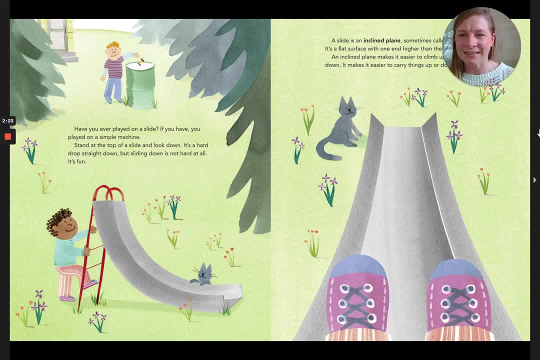 It's a hard drop straight down. but sliding down is not hard at all, It's fun. A slide is an inclined plane, sometimes called a ramp. It's a flat surface with one end higher than the other. An inclined plane makes it easier to climb up and down. It makes it easier to carry things up or 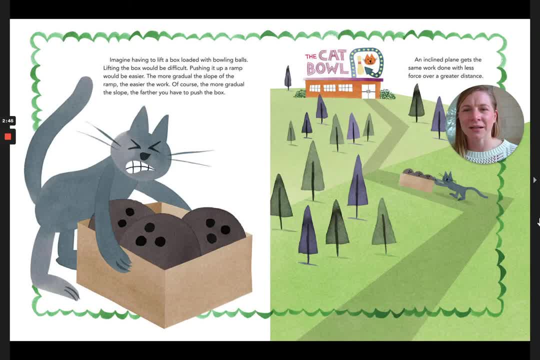 down. Imagine having to lift a box loaded with bowling balls. Lifting the box would be difficult, Pushing it up a ramp would be easier. The more gradual the slope of the ramp, the easier the work. Of course, the more gradual the slope, the further you have to climb. The more you have to climb, the 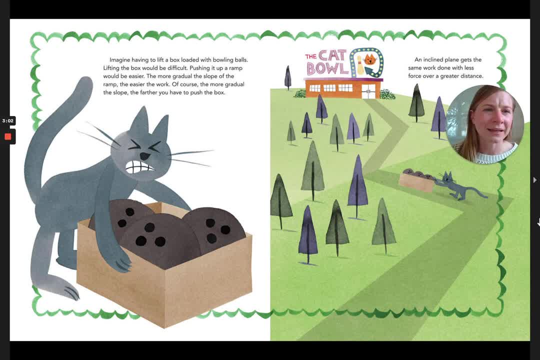 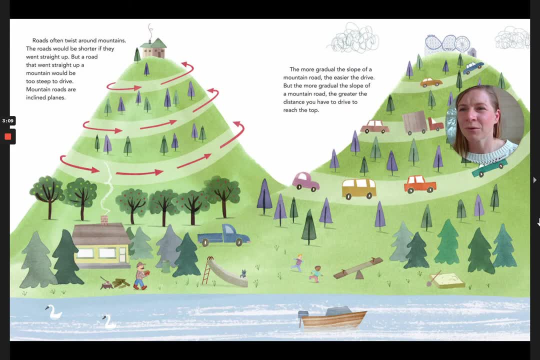 harder. you have to push the box. An inclined plane gets the same work done with less force over a greater distance. Roads often twist around mountains. The roads would be shorter if they went straight up, But a road that went straight up a mountain would be too steep to drive Mountain. 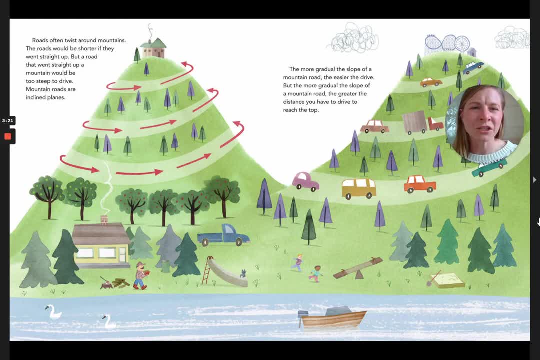 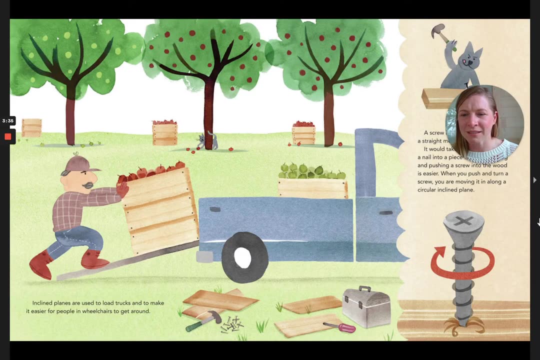 roads are inclined planes. The more gradual the slope of a mountain road, the easier the drive. But the more gradual the slope of the mountain road, the greater the distance You have to drive to reach the top. Inclined planes are used to load trucks and to make it easier for people in wheelchairs to get around. 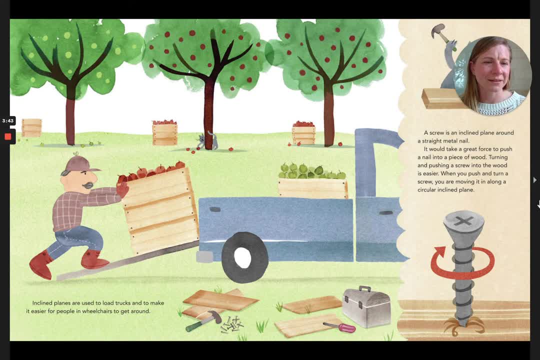 A screw is an inclined plane around a straight metal nail. It would take a great force to push a nail into a piece of wood. Turning and pushing a screw into the wood is easier. When you push and turn a screw, you are moving it in along a circular inclined plane. 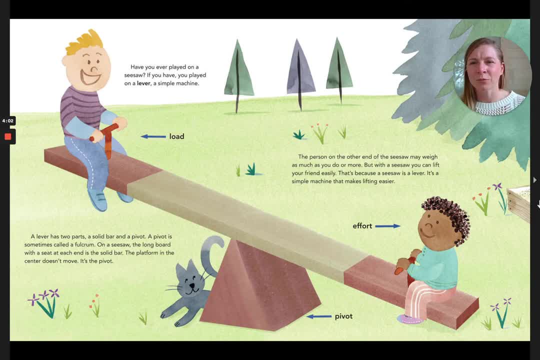 If you have You ever played on a see saw. If you have you played on a lever. A lever has two parts: A solid bar and a pivot. A pivot is sometimes called the fulcrum On a see saw, the long board With a seat at each end. it's a solid bar. 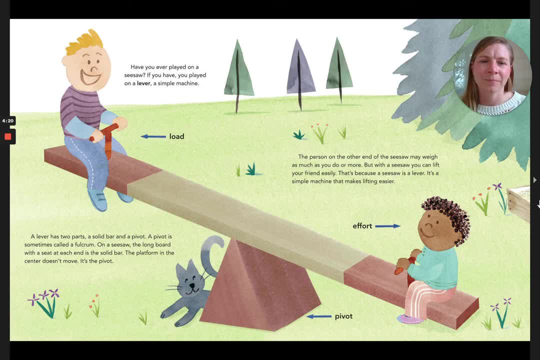 The platform in the center doesn't move. It is the pivot. The person on the other end of that see saw may weigh as much as you do or more, But with a see saw or saw you can lift your friend easily. I neverớ. If it becomes a mat or dice or store. That was really easy to get out on the road. It is the pivot. The good thing about a see saw is that you can hold it by a simple tool in a frying pan, or you can hold the ball and move the other end out easily, or it would just slip. 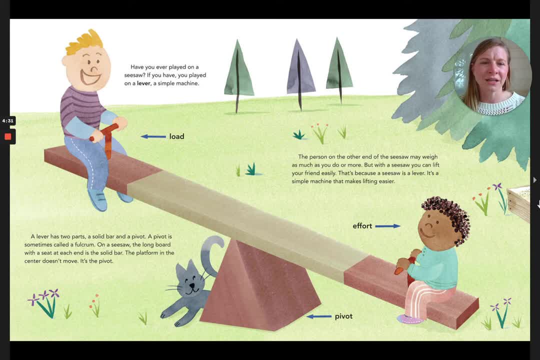 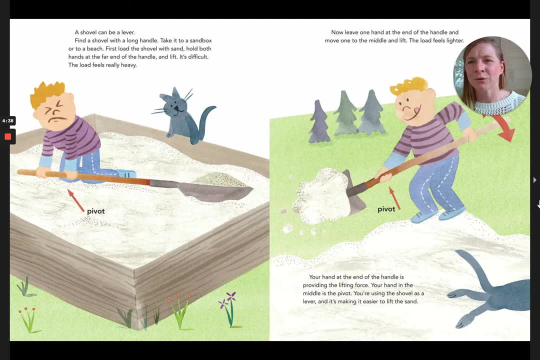 That's because the seesaw is a lever. It's a simple machine that makes lifting easier. A shovel can be a lever. Find a shovel with a long handle, Take it to a sandbox or a beach. First load the shovel with sand, Hold both hands at the far end of the handle and lift. 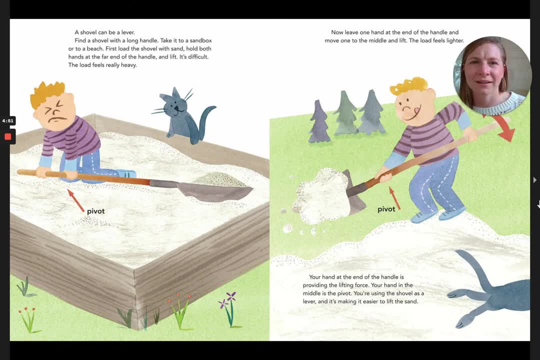 It's difficult. The load feels really heavy. Now leave one hand at the end of the handle and move one to the middle and lift. The load feels lighter. Your hand at the end of the handle is providing the lifting force. Your hand in the middle is the pivot. You're using the. 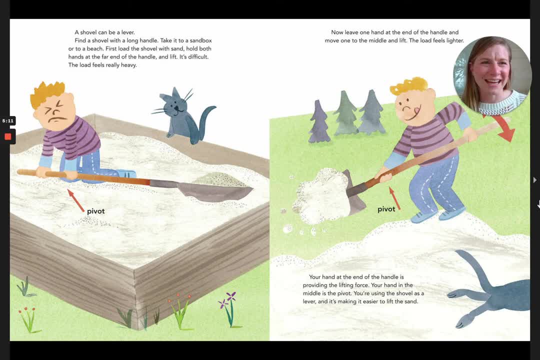 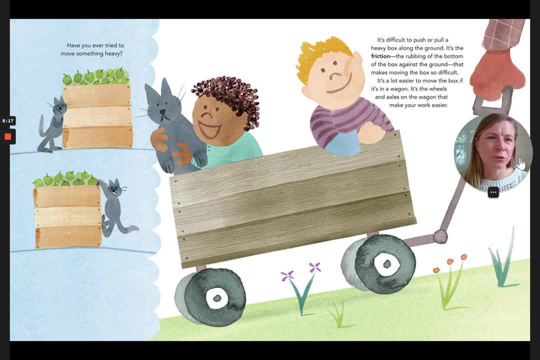 shovel as a lever and it's making it easier to lift the sand. Have you ever tried to move something heavy? It's difficult to push or pull a heavy box along the ground. It's the friction, the rubbing of the bottom of the box against the ground. 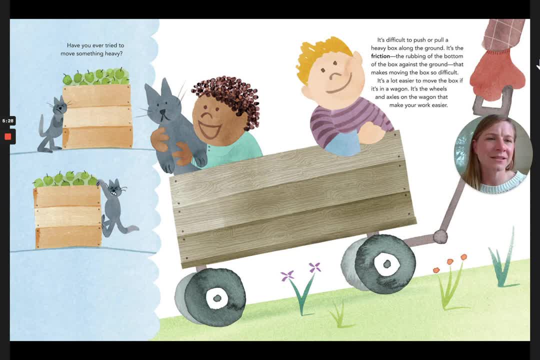 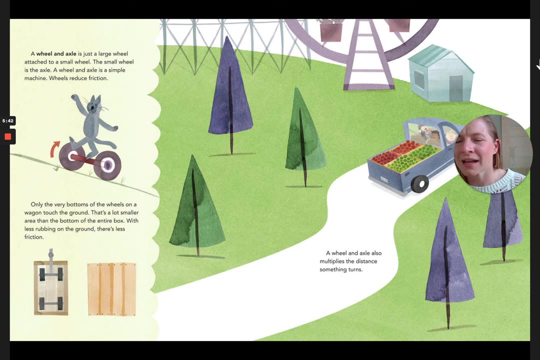 That makes moving the box so difficult. It's a lot easier to move the box if it's in a wagon. It's the wheels and the axles on the wagon that make the work easier. A wheel and an axle is just a large wheel attached to a small wheel. The small wheel is the axle. 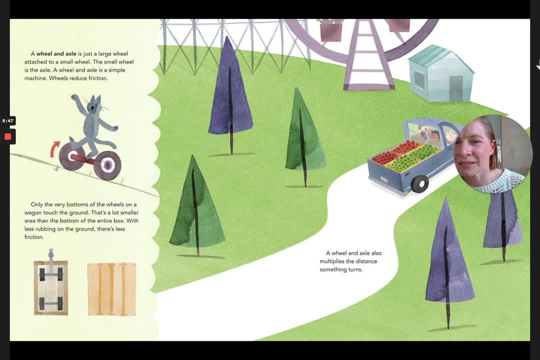 A wheel and axle is a simple machine. Wheels reduce friction. Only the very bottoms of the wheels on a wagon touch the ground. That's a lot smaller area than the bottom of the entire box. With less rubbing on the ground, there's less friction. A wheel and axle: 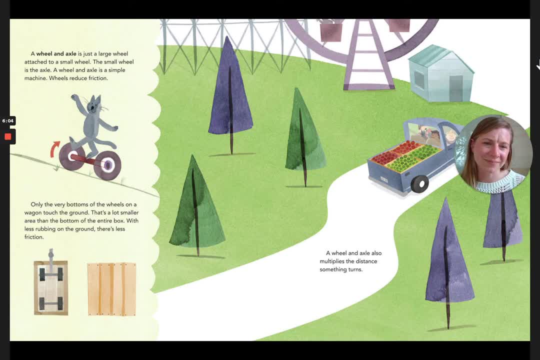 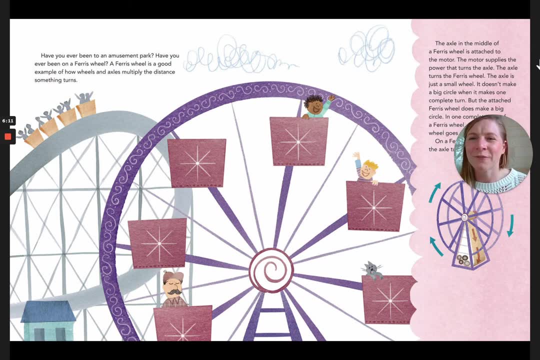 also multiplies the distance. something turns. Have you ever been to an amusement park? Have you ever been on a ferris wheel? A ferris wheel is a good example of how wheels and axles multiply the distance. something turns. The axle in the middle of the ferris wheel is attached to the motor. 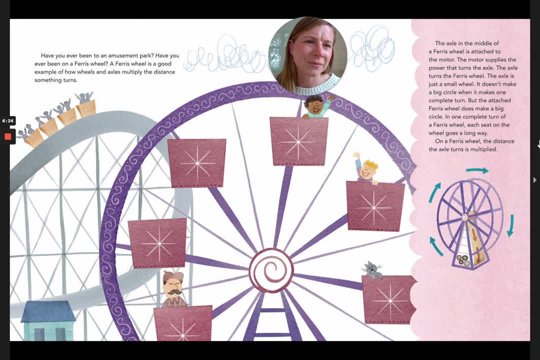 The motor supplies the power that turns the axle. the axle turns the Ferris wheel. The axle is just a small wheel. It doesn't make a big circle when it makes one complete turn, but the attached Ferris wheel does make a big circle In one. 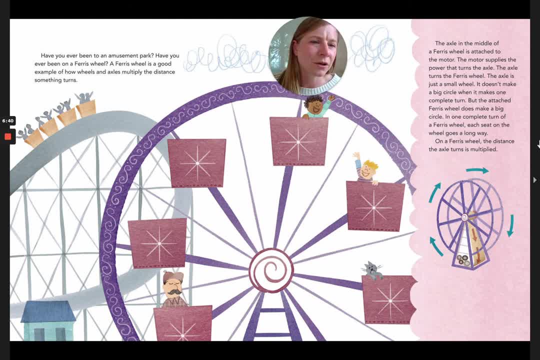 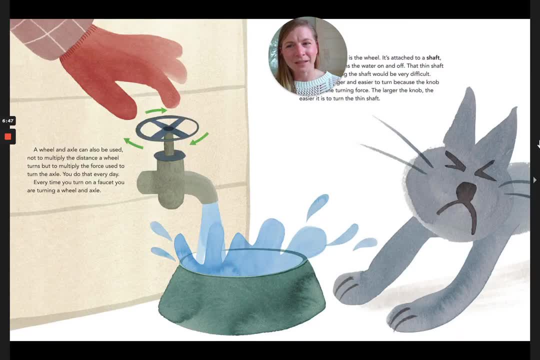 complete turn of the Ferris wheel. each seat on the wheel goes a long way. On a Ferris wheel, the distance the axle turns is multiplied A wheel and an axle can also be used not to multiply the distance of a wheel that the wheel turns, but to multiply the force used to turn. 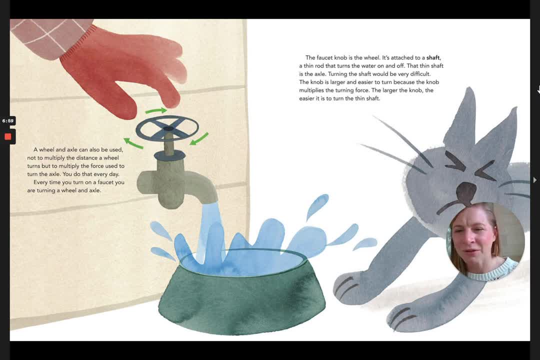 the axle. You do that every day. Every time you turn on a faucet you are turning a wheel and axle. The faucet knob is the wheel. It's attached to a shaft, a thin rod that turns the water on and off. That thin shaft is the axle. Turning the shaft would be very difficult. The knob is 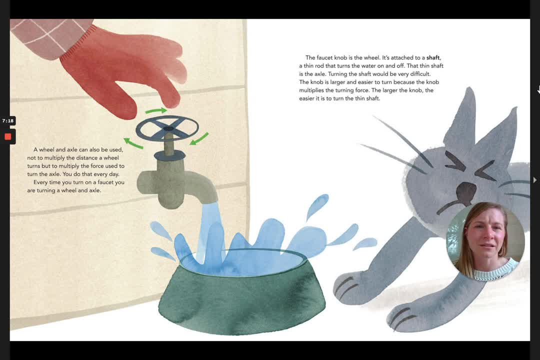 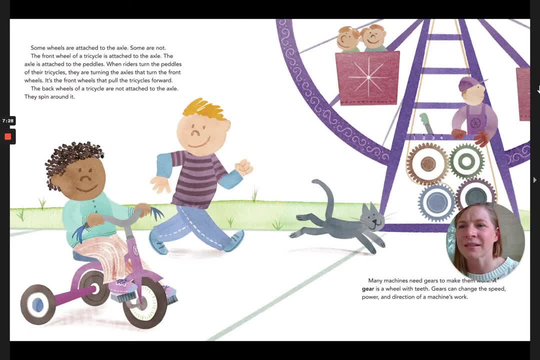 Some wheels are attached to the axle, Some are not. The front wheel of a tricycle is attached to the axle. The axle is attached to pedals. When riders turn the pedals of their tricycles, they are turning the axles that turn the front wheels. It's the front wheels that pull the tricycles forward. 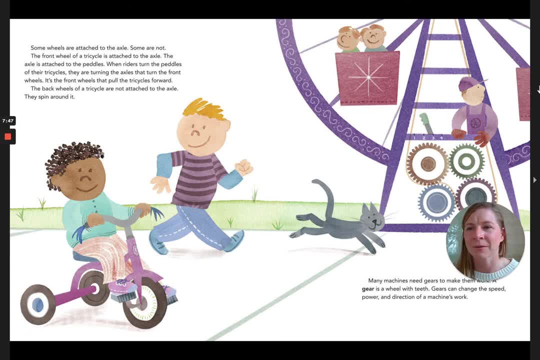 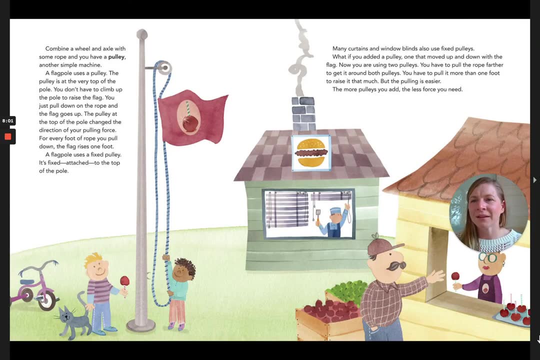 The back wheels of the tricycle are not attached to the axle, They just spin around. Many machines need gears to make them work. A gear is a wheel with teeth. Gears can change the speed, power and direction of a machine's work. Combine a wheel and an axle with some rope and you have a pulley. 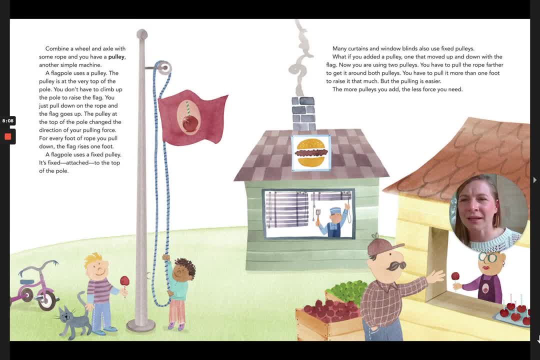 another simple machine. A flagpole uses a pulley. The pulley is at the very top of the pole. You don't have to climb up the pole to raise the flag. You just pull down on the rope and the flag goes up. The pulley at the top of the pole changes the direction of your pulling force. 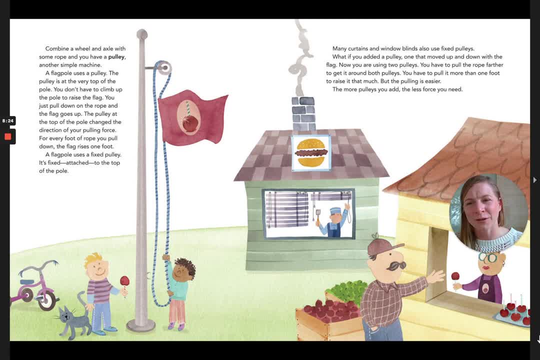 For every foot of rope you pull down, the flag rises one foot. A flagpole uses a fixed pulley. It's fixed attached to the top of the pole. Many curtains and window blinds also used fixed pulleys. What if you added a pulley, one that moved up and down with the flag? 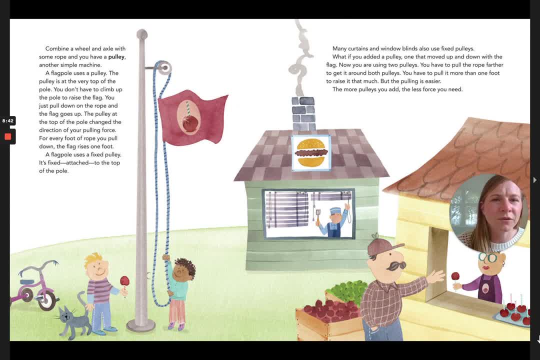 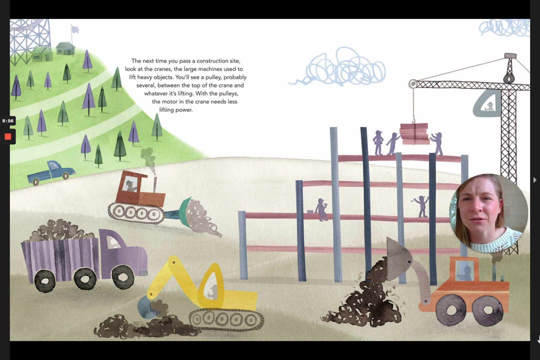 Now you are using two pulleys. You have to pull the rope further to get it around both pulleys. You have to pull it more than one foot to raise it that much. but the pulling is easier. The more you add, the less force you need The next time that you pass a construction site. look at cranes. 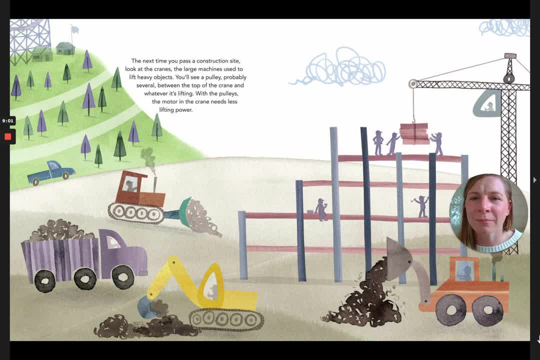 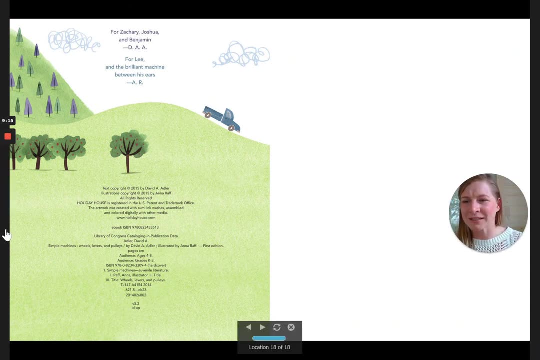 The large machines used to lift heavy objects. You'll see a pulley, probably several, between the top of the crane and whatever it's lifting With the pulleys, the motor in the crane needs less lifting power. That is the end, friends. I hope you understood the simple machines a little bit more based on reading. 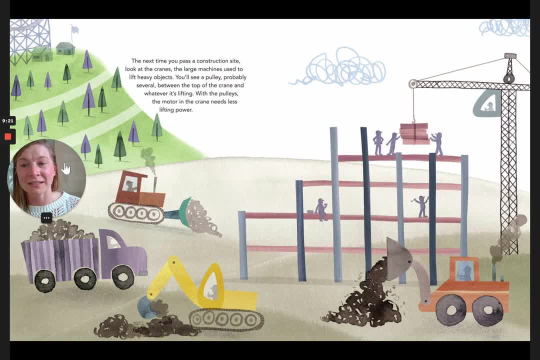 I think it's incredible. I think the pulley is able to do more. I've been doing a lot of work to add the items I need for my cranes- Awesome, See you next week. pulleys, in particular, are extremely incredible that just by adding them, the force becomes less. 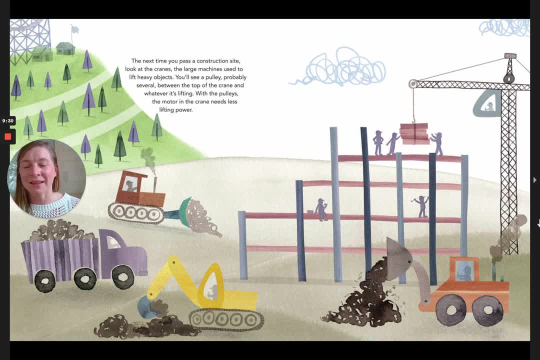 that is needed. all of these simple machines, though, are something that you can go out in your backyard or in your house and find and just kind of play around with and see. you know, how do these simple machines make the work easier, at least from a force standpoint. maybe you have to do more continued. 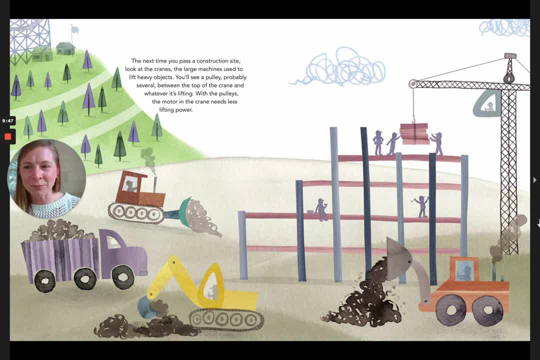 effort, but that's a whole other story. thank you so much for reading this with me, friends. i hope you learned a ton, or even if you learned just a little, that's. that's okay too. have a great day, bye. 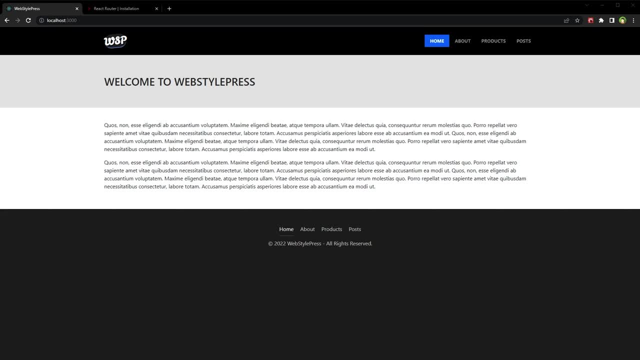 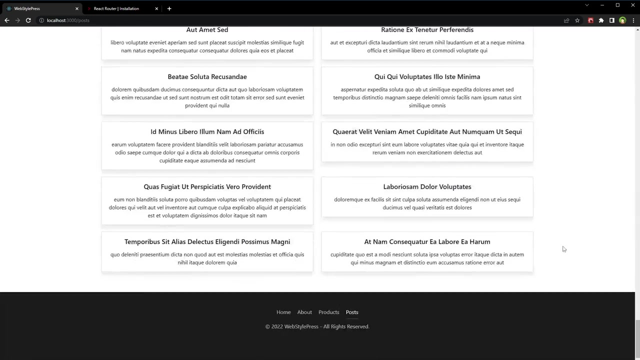 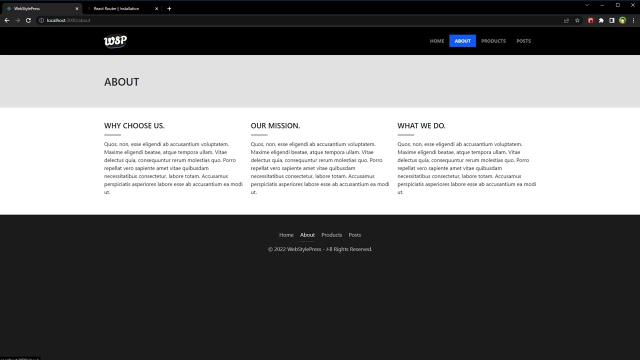 welcome to webstylepress. in this video, we will create a clean, looking, responsive website containing header, footer, navigation, menu pages, product page- single product page- breadcrumbs. header menu- footer menu using react js and latest react router. this is the home page about page posts and this is breadcrumb. we have got header menu, we have got footer menu and we have got. 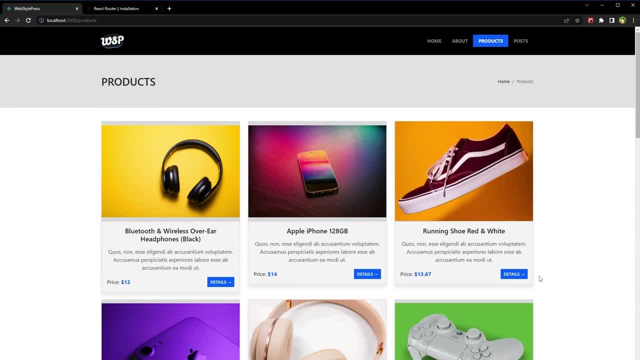 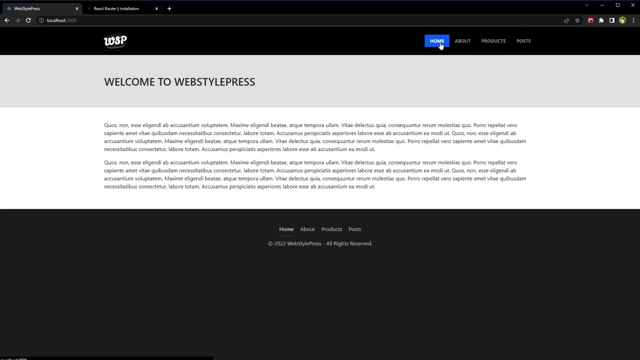 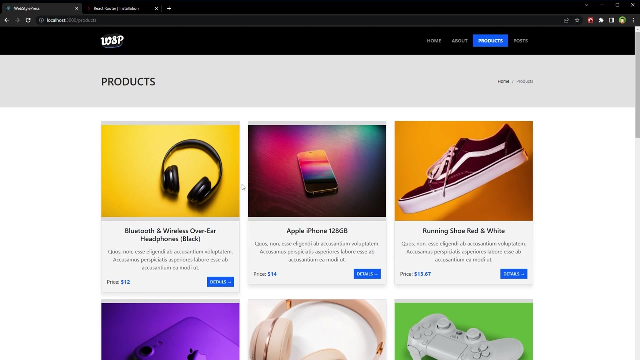 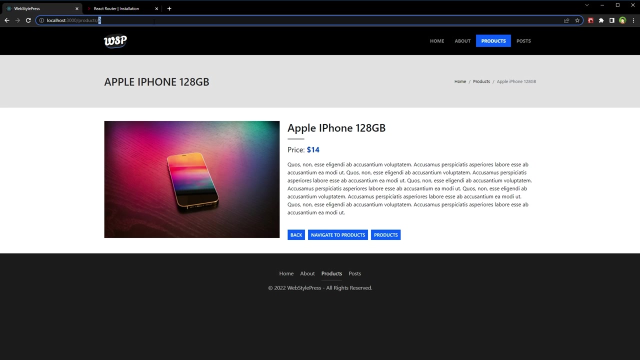 products page and we've got single product page. tutorial shows you how to create routes, use dynamic classes and menus, like you see this active link for the current page. get url parameters to show specific data and all that good stuff, like this product. if i click add this, this is url parameter that we are receiving and we are displaying this data. 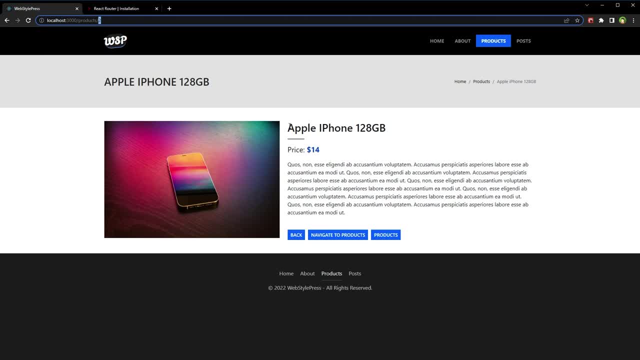 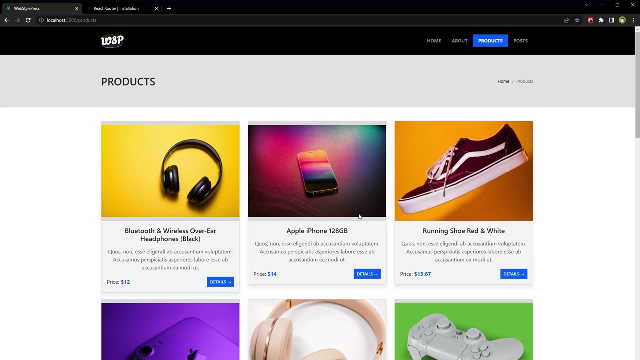 against this id. we can also use permalink like the post name in the url instead of two, but we have used ids. depends on the data type. data will be fetched from javascript object that is in separate file. we can also use an external api for the data for basic styling. 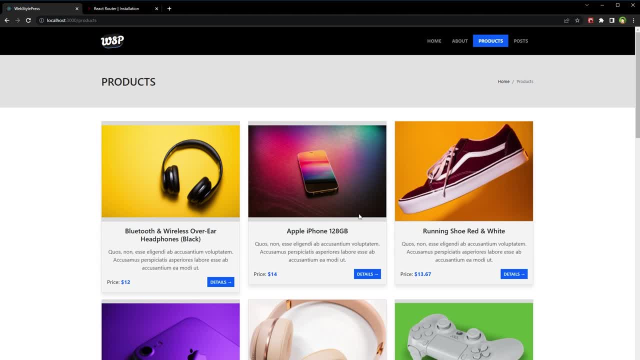 we have used twitter bootstrap. at the end of this tutorial you will be able to understand dynamic routes in react gs, linking different pages in reactjs application, creating menus and more new. react router has smart routing, where router has better algorithm to understand a request to navigate to better result if we go to react router website.